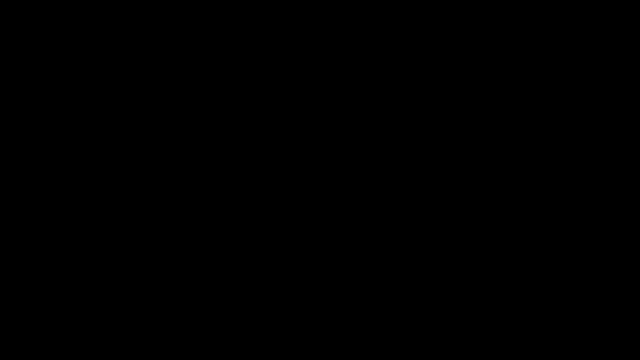 In this video we're going to talk about rotational motion. So what exactly is rotational motion? From the word, you can describe that it's any object that can rotate or spin. So that's rotational motion. It's different from linear motion, where an object simply moves forward. Linear motion and translational motion. 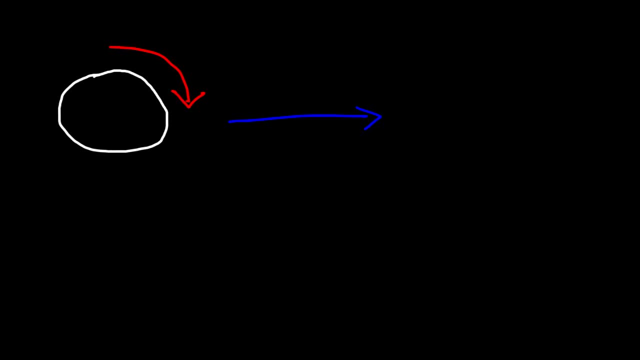 basically means the same thing. Now, so what terms do you need to be familiar with when dealing with rotational motion? Well, in linear motion you have things like position and displacement. For instance, let's say, if this is a number line and an object is currently at position A, So position is basically a. 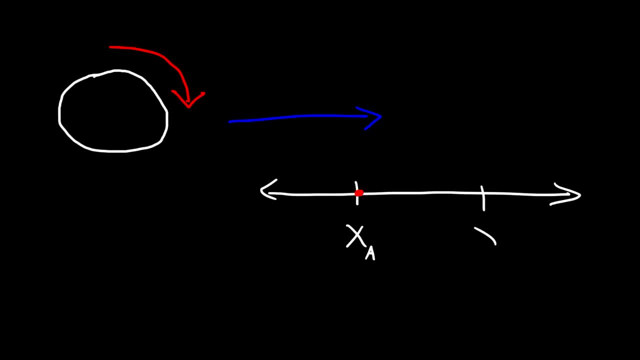 point in space, Displacement is the change in position. Let's say, if the object moves from X A to X B, Then the object's displacement is the difference between XB and XA. It's the final position minus the initial position. that's displacement. Well, for rotational motion we have the same terms. 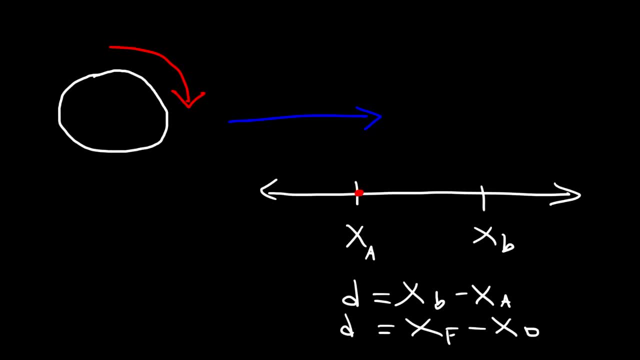 There's angular position and angular displacement. So angular position, just like regular position, is a point on the circle. let's call this point A And let's say, as the wheel spins, point, the object moves from point a. so let's say point B. so this angle. 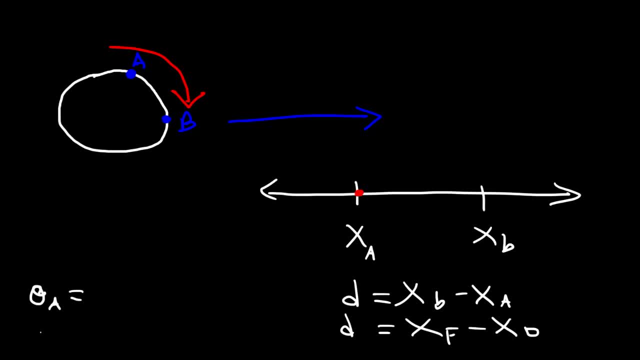 represents the angular position, and this is also the angular position, but the difference between those two points. I guess you can call it Delta theta. this is the angular displacement, it's the difference between those two points in the circle. it's the final angular position minus the initial angular. 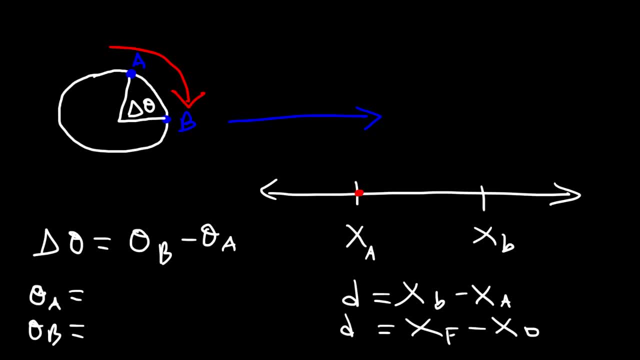 position. so that's angular displacement. now the standard unit for angular displacement is the unit radiance. now you can use degrees or any type of angle measure, but the most common unit that you're going to see is radiance. Now, the next term that you need to be familiar with is angular. 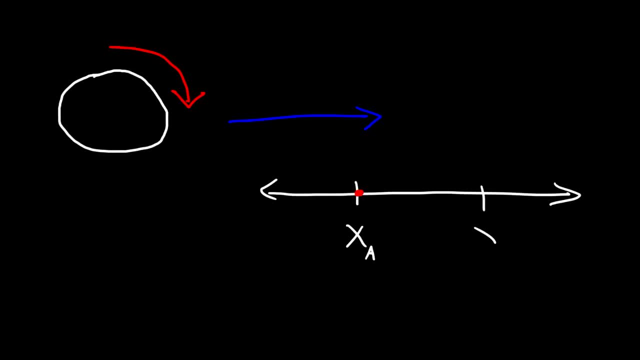 a point-in-space Displacement is the change in position. Let's say, if the object moves from X to X, then the object's displacement is a point-in-space. If the object moves from X to X, then the object's displacement is a point-in-space. 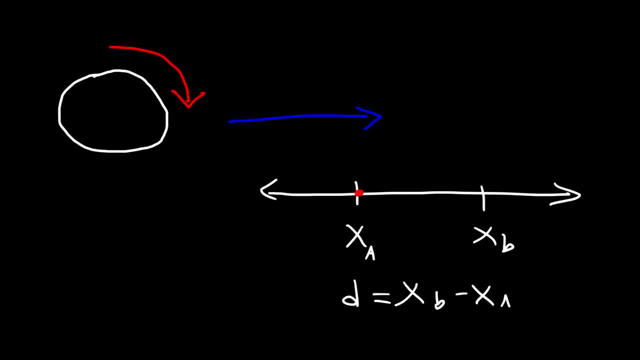 the difference between xb and xa, it's the final position minus the initial position. that's displacement. well, for rotational motion we have the same terms. there's angular position and angular displacement. so angular position, just like regular position, is a point on the circle. let's call this. 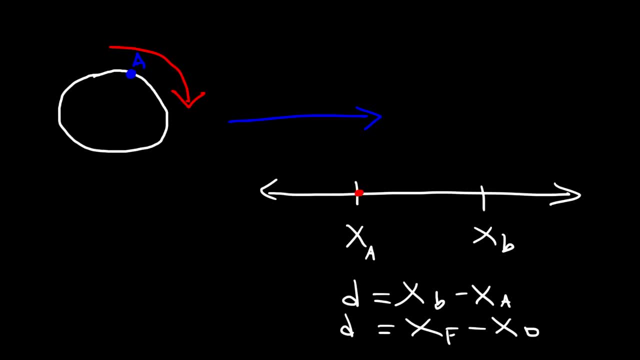 point a and let's say, as the wheel spins, point, the object moves from point a to, let's say, point b. so this angle represents the angular position and this is also the angular position, but the difference between those two points. i guess you can call it delta, theta. this is the angular 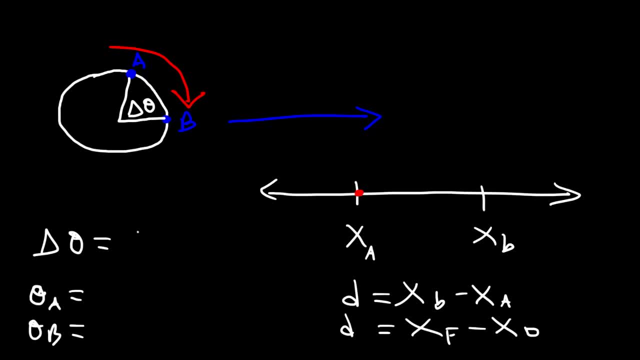 displacement it's the difference between those two points in the circle. it's the final angular position, the minus the initial angular position. so that's angular displacement. now the standard unit for angular displacement is the unit radians. now you can use degrees or any type of angle measure, but the most common unit that you're going to see is radians. 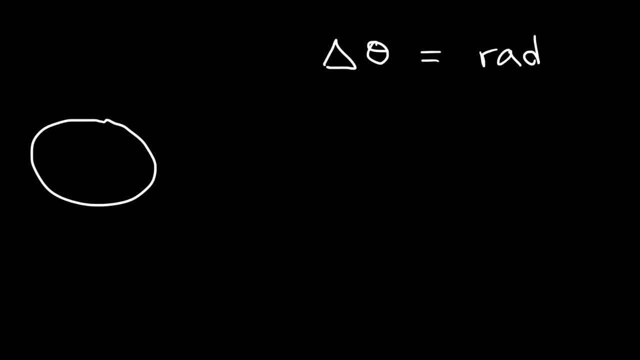 so now the next term that you need to be familiar with is angular velocity. angular velocity tells you how fast an object is spinning on a circle, whereas linear velocity tells you how fast it's moving forward. so the average linear velocity, or let's say average linear speed, is distance divided by time. 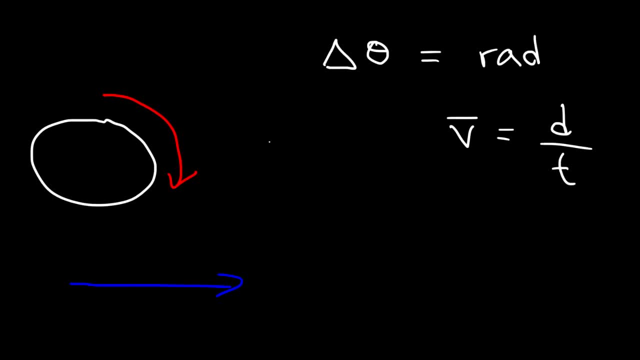 velocity is really displacement over time, but the units will still be meters per second. now, angular velocity, which is represented by the symbol omega. this is going to be average angular velocity. it's equal to the angular displacement divided by the time and, as you can see, the equations are very similar. 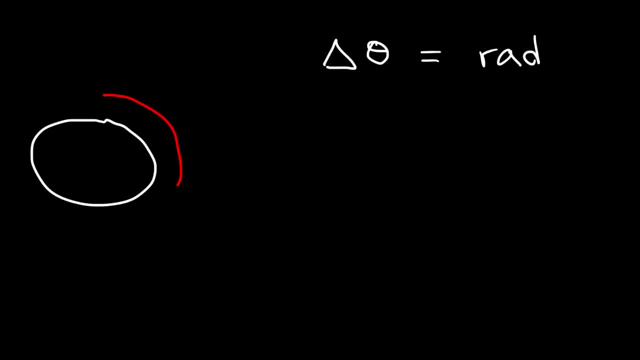 velocity. Angular velocity tells you how fast an object is spinning on a circle, whereas linear velocity tells you how fast it's moving forward. So the average linear velocity, or let's say average linear speed, is distance divided by time. Velocity is really displacement over time, but the units will still be meters. 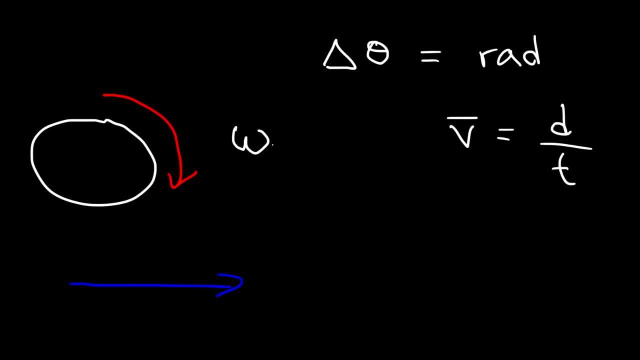 per second. Now angular velocity, which is represented by the symbol Omega. this is going to be average angular velocity. it's equal to the angular displacement divided by the time And, as you can see, the equations are very similar. So for average angular velocity, it's equal to the angular displacement divided by the time And, as you can see, the equations are very similar. So for average, 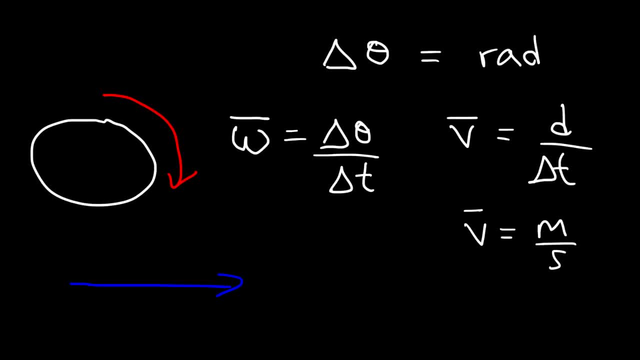 velocity we have units such as meters per second and for average angular velocity it's radians per second. So here this is going to be displacement over time to get velocity and to get angular velocity, it's angular displacement over time. Now the equation that connects linear velocity to angular velocity is: 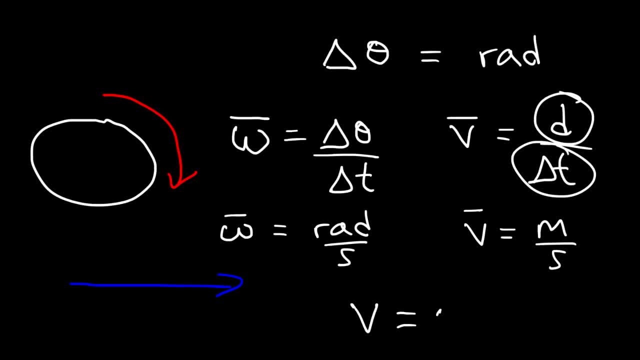 this equation, Linear velocity is equal to omega times R, So whenever you have an object spinning, the angular speed is the same everywhere on a circle. However, the linear speed is not the same, So let me give you an example that will illustrate this. So let's say this is the center of 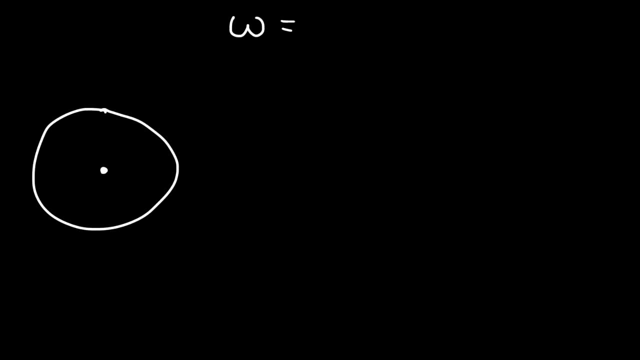 the circle, and this circle is spinning at five radians per second. So let's say this is point A and this is point B. Let's move point B to this position. So which one has the greater angular velocity, Point A or point B? Now 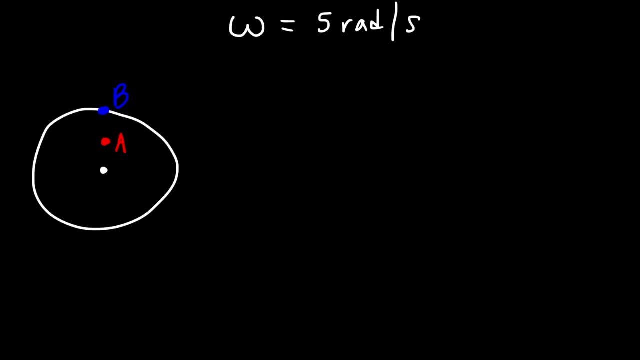 because the wheel is spinning at one angular speed. every point on this wheel will travel at that same speed. It's going to rotate at that same rate. so the angle of velocity of a is equal to the angle of velocity of point B. they're going to rotate at the same rate. now what about? 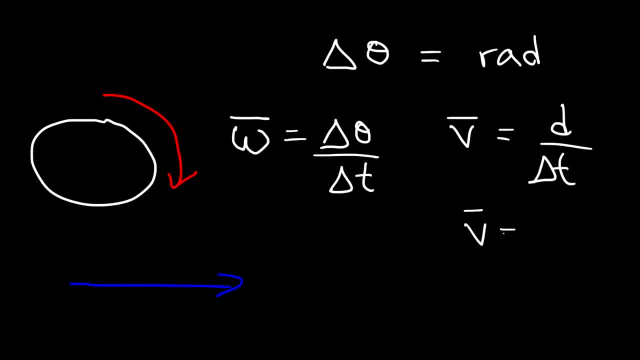 so for average velocity we have units such as meters per second and for average angular velocity its radians per second. so here this is going to be displacement over time to get velocity and to get angle velocity it's angular displacement over time. now the equation that connects linear velocity to angular velocity is this: 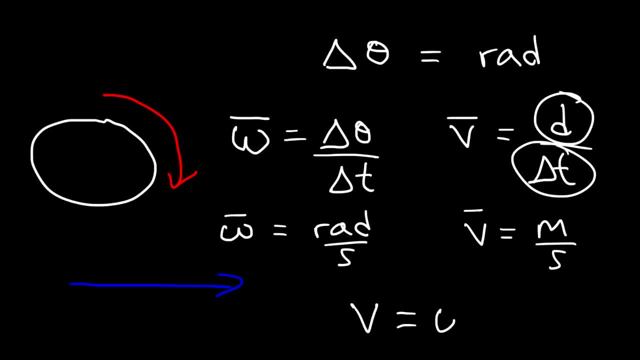 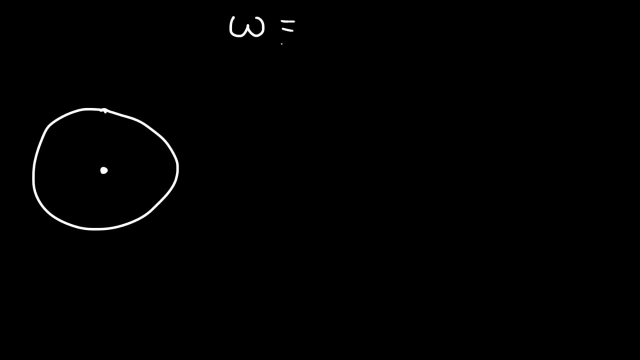 equation, linear velocity is equal to Omega times R, so whenever you have an object spinning, the angular speed is the same. everywhere on a circle, however, the linear speed is not the same, so let me give you an example that will illustrate this. so let's say this is the center of the circle and this circle is 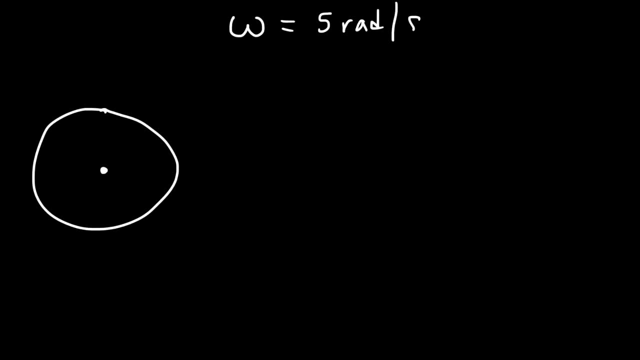 spinning at 5 radians per second. so let's say this is point a and this is point B. let's move point B to this position. so which one has the greater angular velocity, point a or point B? now, because the wheel is spinning at one angular speed, every point on this wheel will travel at that same speed. it's 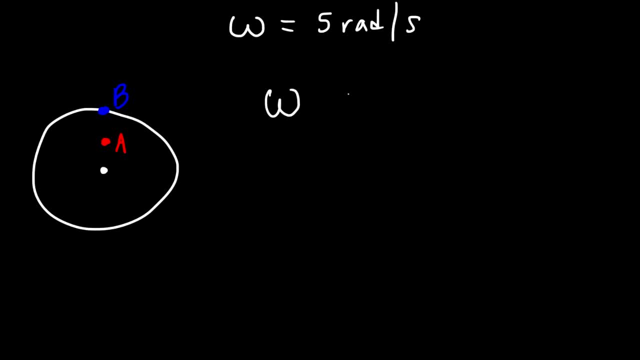 going to rotate at that same rate. so the angular velocity of a is equal to the angular velocity of point B. they're going to rotate at the same rate. now, what about the linear velocity? is it the same or is it different? now they're all spinning at the same rate, but point a has a shorter distance to travel point B. 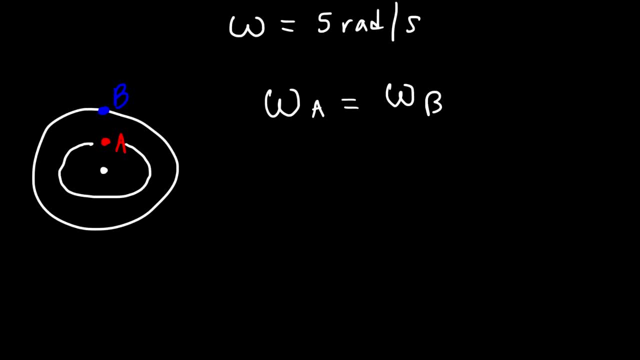 has to travel a longer distance and, in order to spin at the same rate, B has to travel faster than a. so, therefore, the linear speed of point B is greater than the linear speed of point a, and there's an equation that we can use. it's this one: V is equal to Omega times R, so as R increases, the 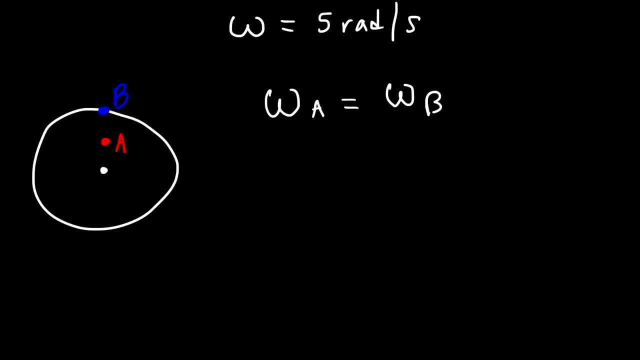 the linear velocity. is it the same or is it different? now they're all spin at the same rate, but point a has a shorter distance to travel. point B has to travel a longer distance and, in order to spin at the same rate, B has to travel faster. 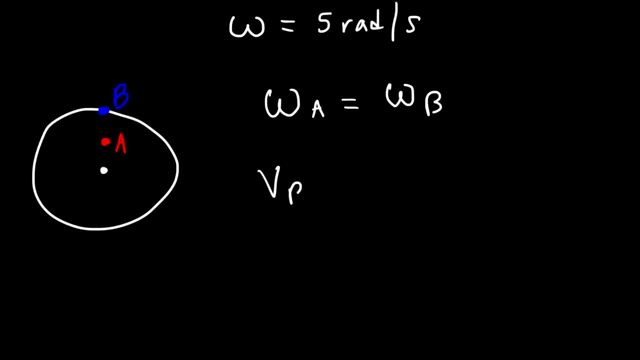 than a. so therefore, the linear speed of point B is greater than the linear speed of point a, and there's an equation that we can use. it's this one: V is equal to Omega times R, so as R increases, the linear velocity will increase. so notice that our a is less than our B. 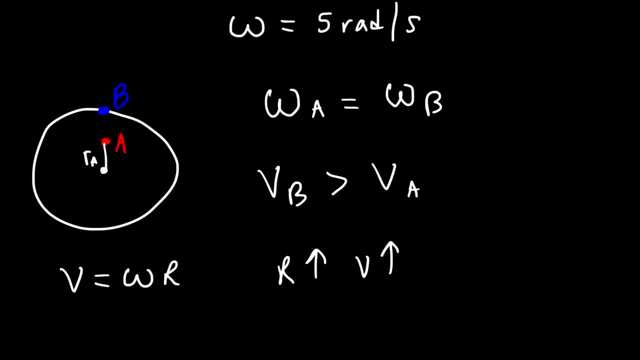 so that's one reason why the linear velocity of B is greater than the linear velocity of point a. now there's some other terms that you need to know, and that is the period and the frequency. the period is the time it takes to complete one cycle. so if you have the total time and the number of cycles that I will 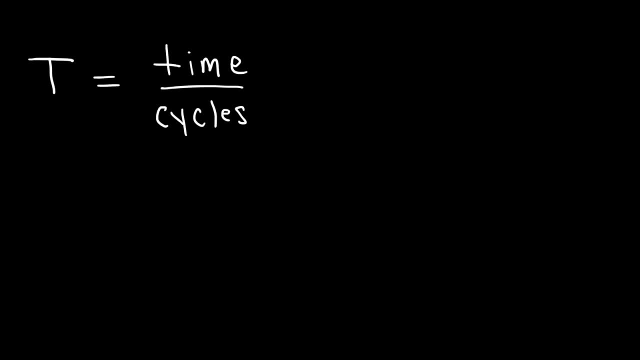 make or rotations. if you divide these two, you're going to get the time it takes to make one complete cycle or one full rotation around the circle. frequency is the reciprocal of period. it's the number of cycles that occurs per second. so if you have the number of 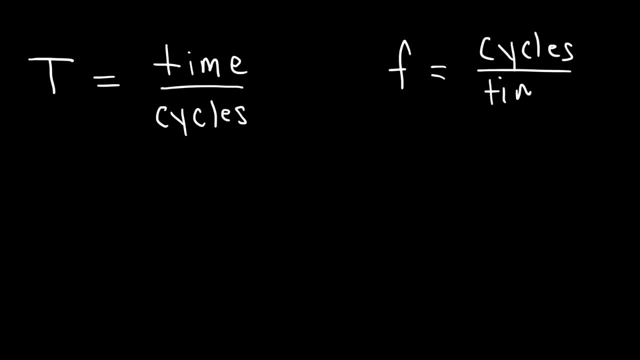 cycles and you divide it by the time. this will give you the frequency. so the unit for period is the seconds, but it's really seconds per cycle or seconds per revolution. the unit for frequency is Hertz or one over seconds. now periods is one divided by the frequency. you can also calculate the angular velocity if 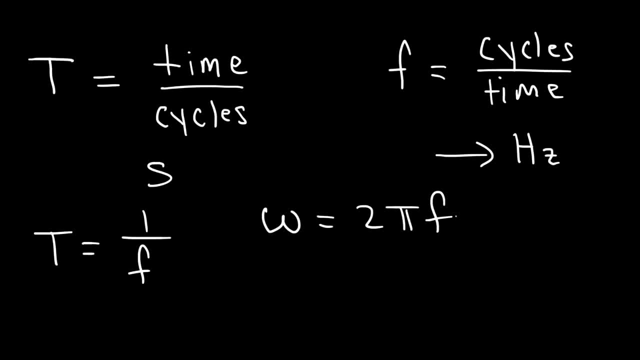 you know the frequency. the angular velocity is equal to 2 pi f. so this is one equation that you want to commit to memory and you also want to know this one as well. now, if you have the period and you want to calculate the angular speed, you can use this equation. Omega is equal to 2 pi divided by T. 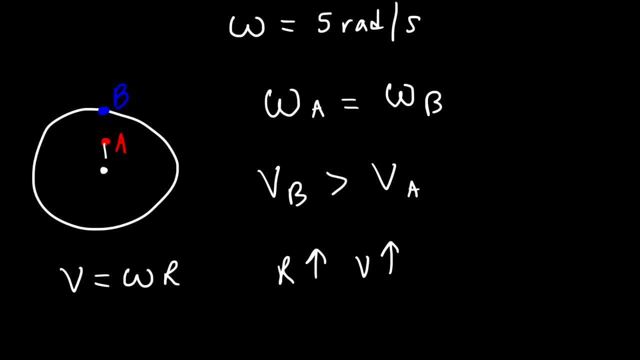 linear velocity will increase. so notice that our a is less than our B. so that's one reason why the linear velocity of B is greater than the linear velocity of point a. now there's some other terms that you need to know, and that is the period and the frequency. the period is the time. 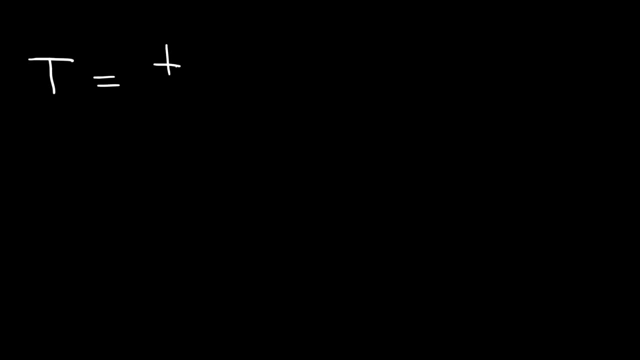 it takes to complete one cycle. so, if you have the total time and the number of cycles that a will make, or rotations, if you divide these two, you're gonna get the time it takes to make one complete cycle or one full rotation around a circle. frequency is the reciprocal of period. it's the number of cycles that occurs per. 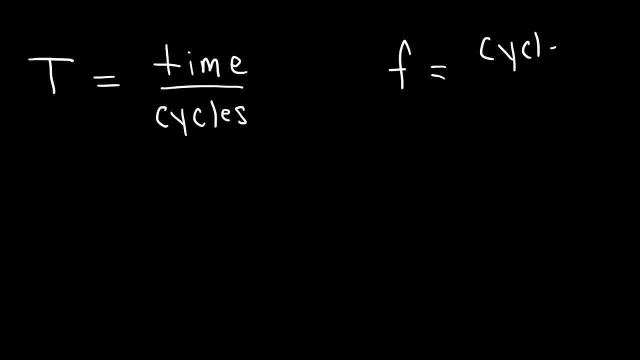 second. So if you have the number of cycles and you divide it by the time, this will give you the frequency. So the unit for period is the seconds, but it's really seconds per cycle or seconds per revolution. The unit for frequency is hertz or 1 over seconds. 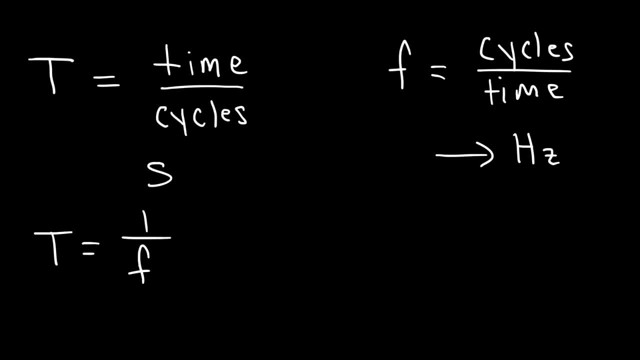 Now, period is 1 divided by the frequency. You can also calculate the angular velocity. if you know the frequency, The angular velocity is equal to 2 pi f. So this is one equation that you want to commit to memory, And you also want to know this one as well. Now, if 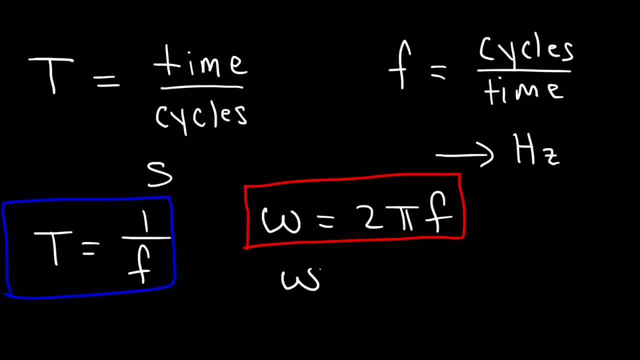 you have the period and you want to calculate the angular speed, you can use this equation: Omega is equal to 2 pi divided by t. So make sure you know those three equations that can relate angular velocity with period and frequency. Now the next thing that we need to talk about is angular acceleration and linear acceleration. 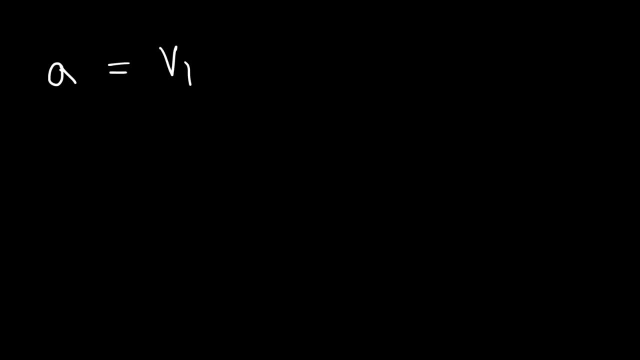 So linear acceleration is the change in velocity divided by the change in time. So this is average linear acceleration. The average angular acceleration is equal to a very similar equation. It's the change in angular velocity by the change in time. The units for linear acceleration is meters per second. 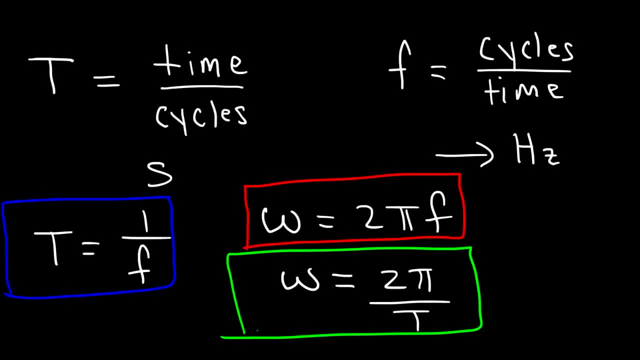 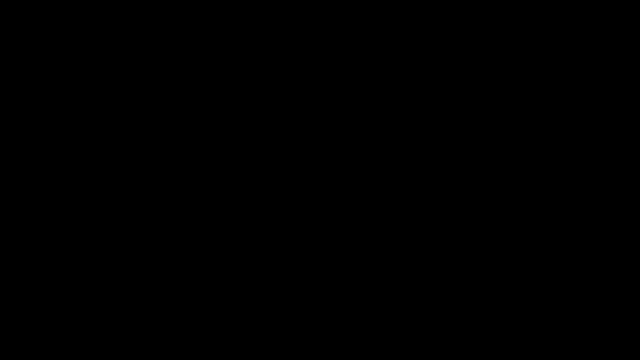 so make sure you know those three equations that can relate angular velocity with period and frequency. now the next thing that we need to talk about is angular acceleration and linear acceleration. so linear acceleration is the change in velocity divided by the change in time. so this is average linear 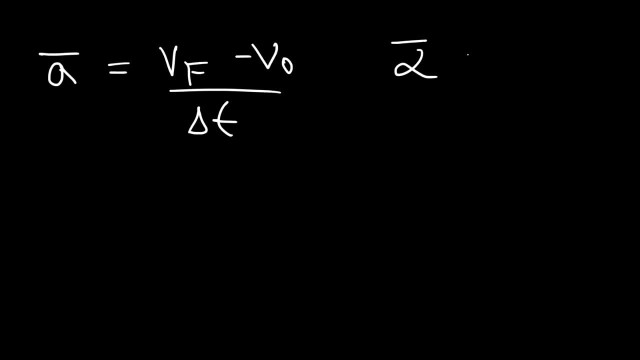 acceleration. the average angular acceleration is equal to. a very similar equation is the change in angular velocity divided by the change in time. the units for linear acceleration is meters per second squared. for angular acceleration its radians per second squared. at least that's the standard unit. it's rare that. 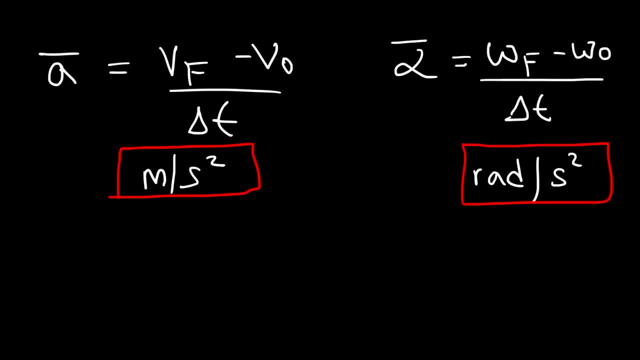 you'll see degrees per second squared, but that would still be a form of angular acceleration. but this is the most common unit. now, whenever you have an object moving in circular motion, there's different types of accelerations that you need to be familiar with. so if the object has any kind of speed, if it's moving around a 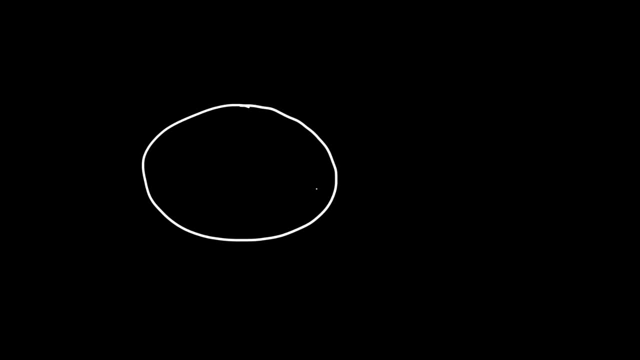 circle. it's going to have a centripetal acceleration and that centripetal acceleration points towards the center of the circle. the centripetal acceleration is equal to the linear speed squared divided by the radius of the circle, and we know that V is equal to Omega R. so this in trip vier's: 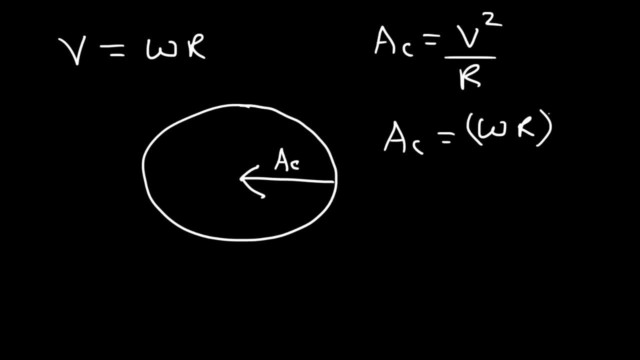 salvations gonna be omega R squared divided by R, so you can cancel one of the ours. so just to take it one step at a time. once you square Omega R, you're going to have for Omega squared times. R squared, which is our times are, I think, a. 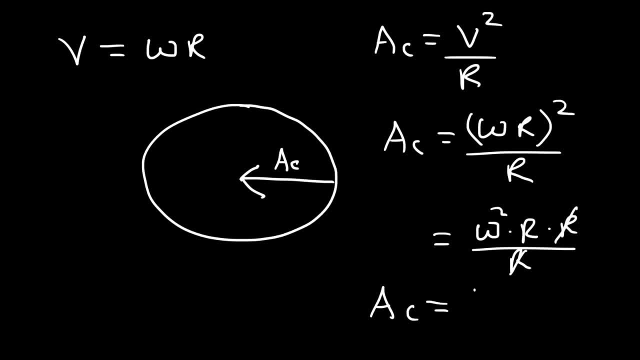 cancel one of these. so the centripetal acceleration is omega squared times r, So that's the acceleration that points towards the center of the circle. So if an object is moving with constant speed around a circle, the only acceleration it has is the centripetal acceleration, also known as the radial acceleration. 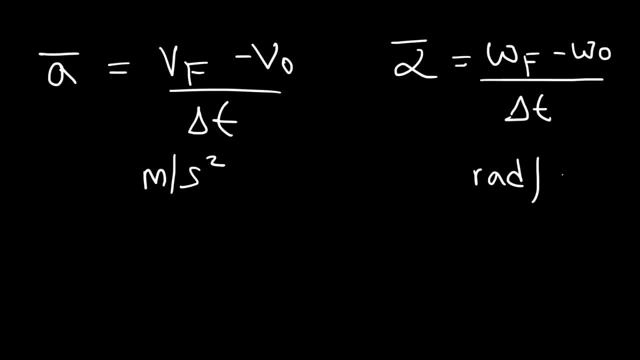 squared. For angular acceleration it's radians per second squared. at least that's the standard unit. It's rare that you'll see degrees per second squared, but that would still be a form of angular acceleration, but this is the most common unit Now whenever you have an object moving in circular motion. 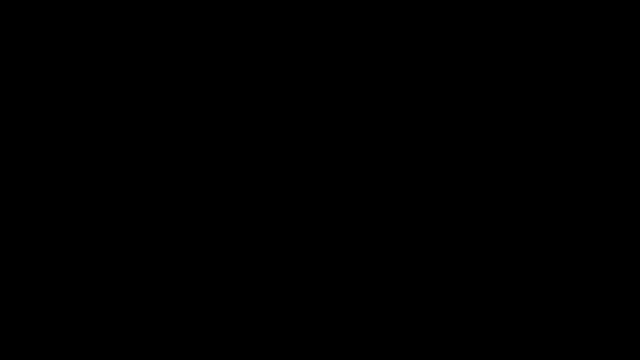 there's different types of accelerations that you need to be familiar with. So if the object has any kind of speed, if it's moving around a circle, it's going to have a centripetal acceleration and that centripetal acceleration points towards the center of the circle. The centripetal 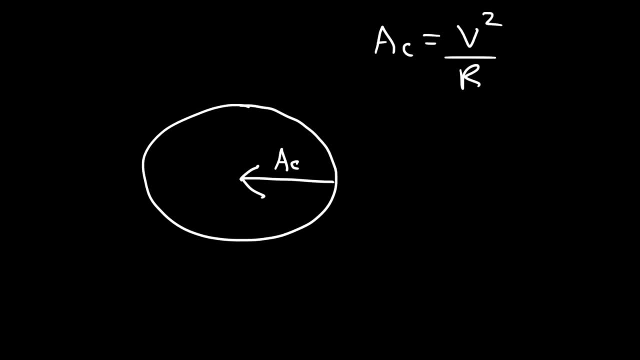 acceleration is equal to the linear speed squared divided by the radius of the circle, and we know that V is equal to Omega R. It's so the centripetal acceleration is going to be Omega R squared divided by R, So you can cancel one of the R's. So just to take it one step at a time. 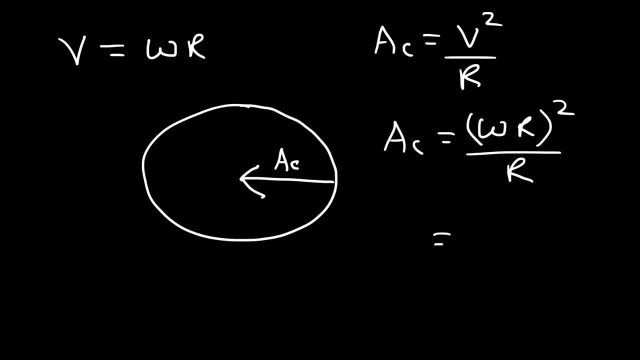 once you square Omega R, you're going to have Omega squared times R squared, which is R times R, And then you can cancel one of these. so the centripetal acceleration is Omega squared times R. So if we have this UV axis interval, I'm just going to stick with. watch this. 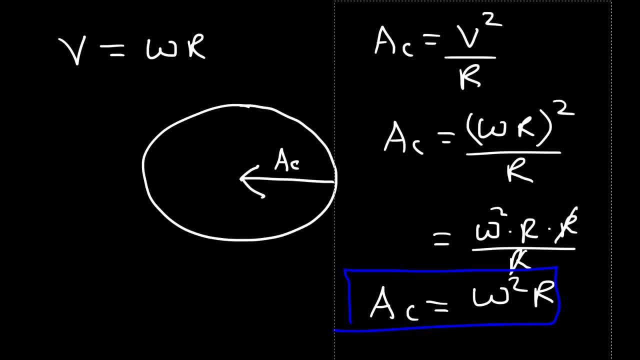 iant ungefähr region. and then I thought, okay, we've got to lower that a bit. It's called it, But if we're going to have a notine, it's a centripetal acceleration. So if there's some kind of speed bets that are going up or vice versa, 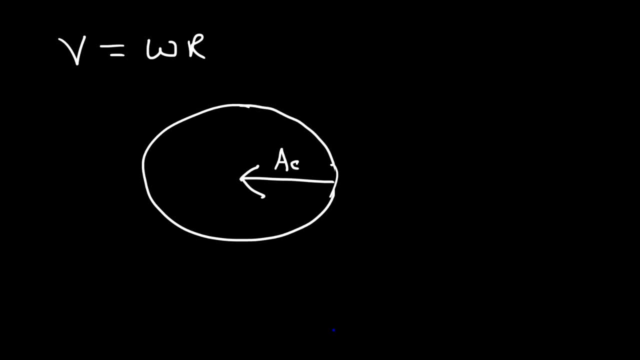 what's we're going to do is we're going to have some kind of acceleration that points towards the center of the circle. Let me avoid doing this a little bit longer here. Oh, here we go. it's moving with constant speed. Now, what if it's not moving with constant speed? 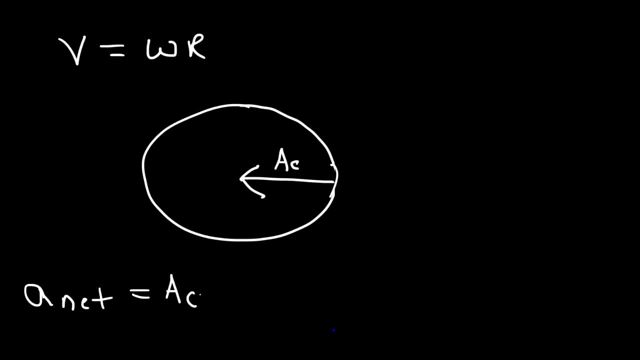 What if it's accelerating around a circle? So then it's going to have a tangential acceleration and the tangential acceleration is equal to the angular acceleration times, R. And we also found the tangential acceleration using this equation: it's the change in velocity divided by the change in time. 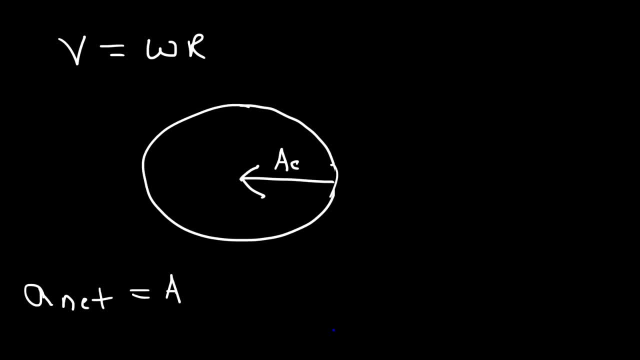 So the net acceleration of the object will equal ac if it's moving with constant speed. Now, what if it's not moving with constant speed? What if it's accelerating around a circle? So then it's going to have a tangential acceleration and the tangential acceleration is equal to. 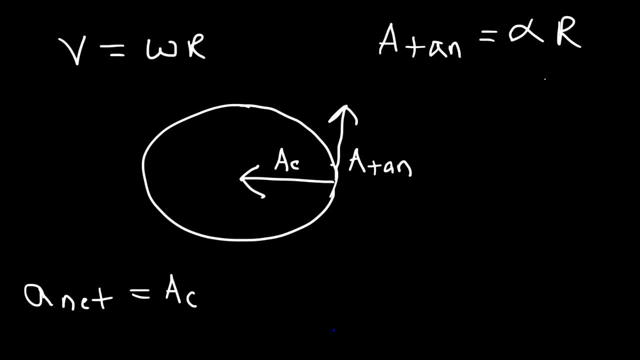 the angular acceleration times r, and we also found the tangential acceleration using this equation: It's the change in velocity divided by the change in time. Now notice that these two vectors, they're perpendicular to each other. So if we have the centripetal acceleration going this way, and this is the tangential, 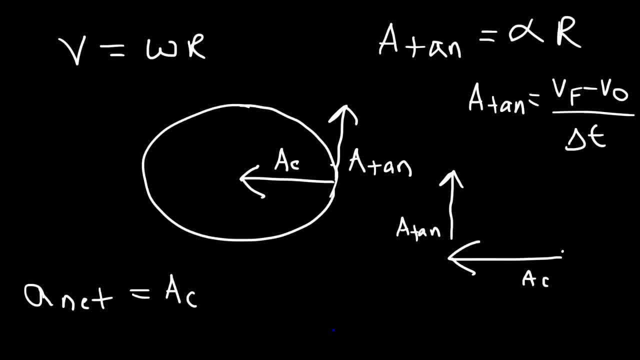 acceleration. Therefore the net acceleration of the object is equal to the angular acceleration times r. So when we move the object at this instant, it's going in the northwest direction. So when the object is not moving with constant speed around a circle, the net acceleration 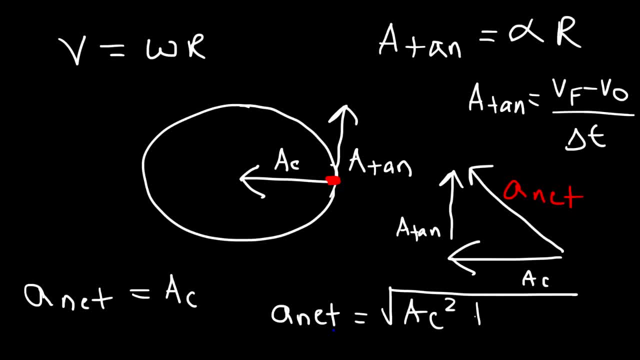 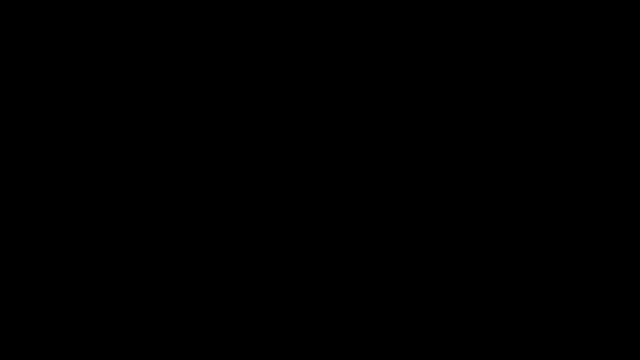 is the vector sum of the centripetal acceleration and the tangential acceleration. So basically it's the hypotenuse of the right triangle. So it's tricky to calculate because it's not vertical. Let's do this again, Bring it to our current position. this is our我覺得. this is what we're going to do. The tensileix style, It's gonna go in here right at the in behavior. This will give us notorious acceleration. This is a speed. 북 التي, Shelby Tten enlai r verbal society morning commentary. 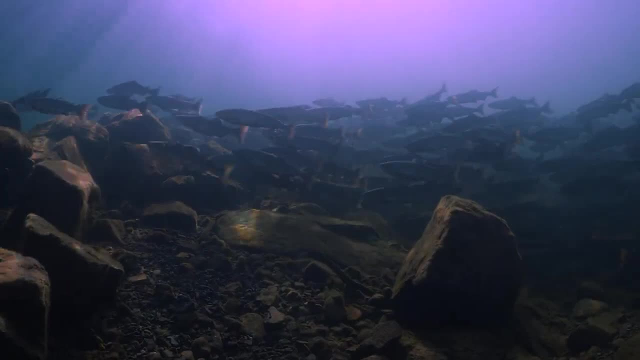 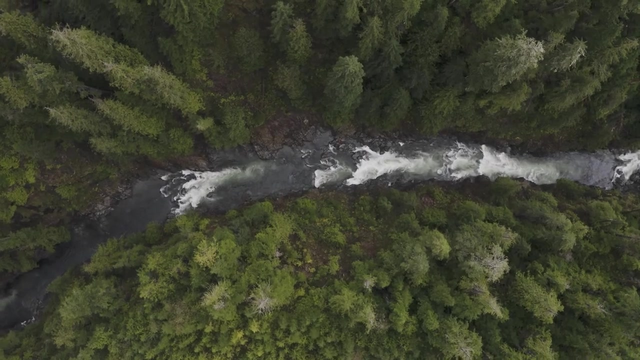 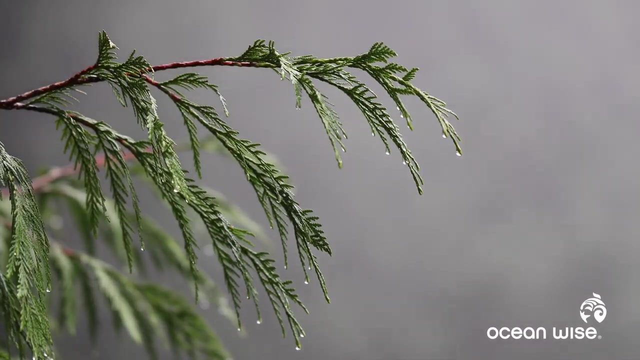 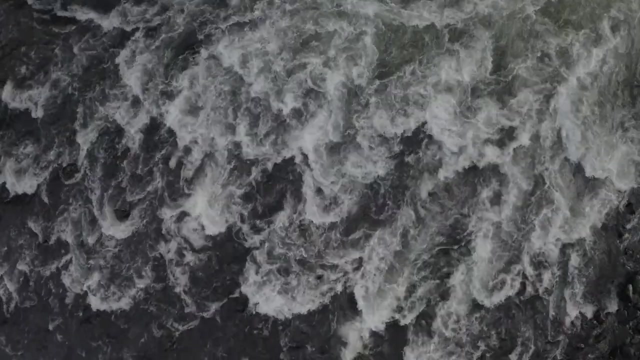 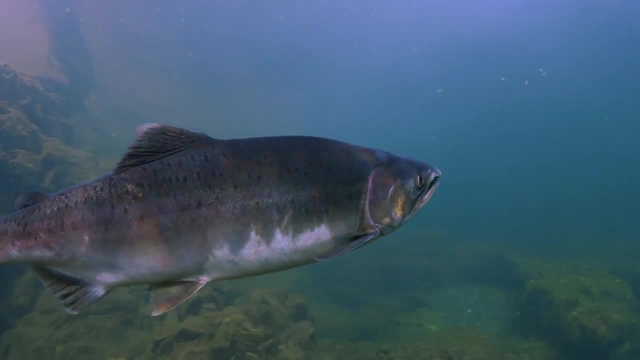 After spending several years in the open ocean feeding and growing, these salmon are returning home, And what they're bringing back benefits an entire ecosystem. Along the west coast of North America, heavy autumn rains have transformed small streams into roaring rivers, allowing millions of salmon to migrate inland in order to spawn.